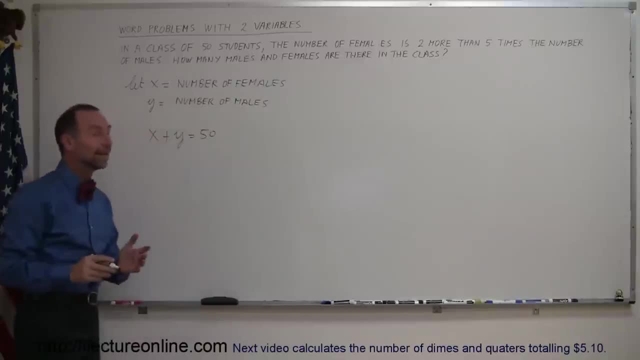 The number of females plus the number of males must add up to 50. And then it says that the number of females- and since the number of females is defined as Y, we can then say that Y is equal to two more plus two, then five times the number of males. 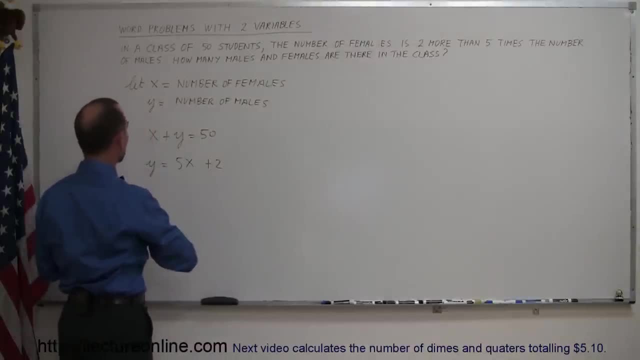 So five times the number of males. So five times the number of males, And X- oh wait, a minute, I think I just got that wrong- Y represents, see, that's why it's so important to very carefully define your variables. 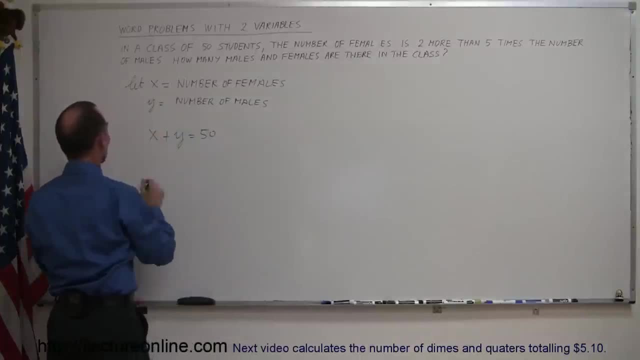 It says the number of females, and the number of females is X. So X is equal to two more plus two, five times the number of males, and the number of males is Y. So five times Y plus two. Notice, if I had not very well defined my X and Y, I probably would not have caught my mistake. 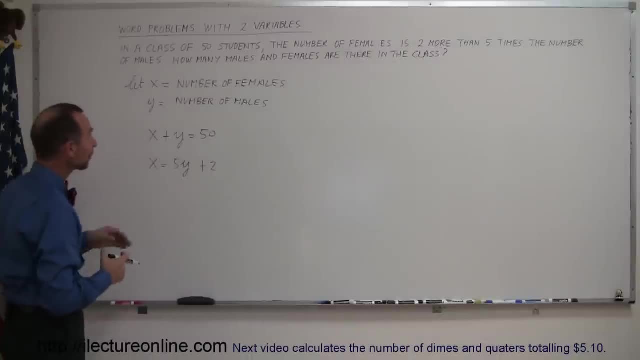 and you would not have gotten the problem, or I would not have gotten the problem right. So that shows how important it is to define your variables carefully. So let's recap quickly: In a class of 50 students, so X plus Y must be 50.. 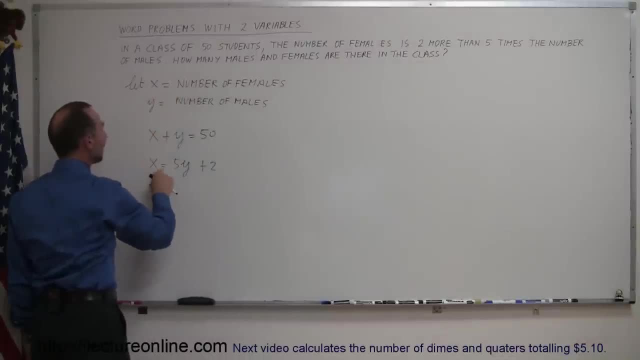 And the number of females, which is defined by X, is equal to two more plus two, then five times the number of males. so plus two added to five times Y, where Y is the number of males. And now we're good to go. 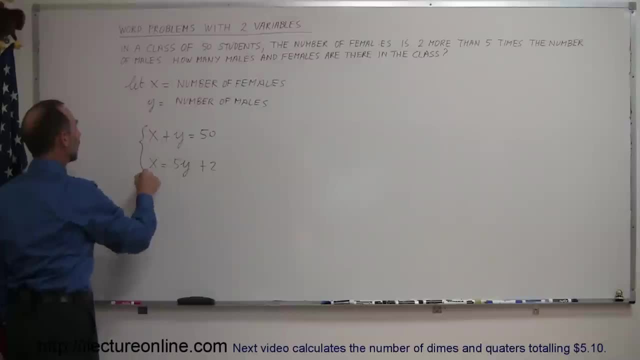 So how do we solve these two equations? Well, we can already use this equation right here, because it's already solved: X in terms of Y. We substitute that into the other equation. So instead of X we write 5Y. so that's this equation, right here. 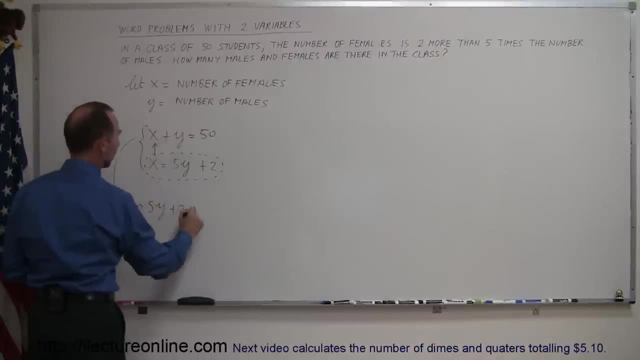 5Y plus two instead of the variable. X plus Y equals 50. So notice that this X is replaced by 5Y plus two. Now we put all the Y's in one place, all the numbers on the other place. 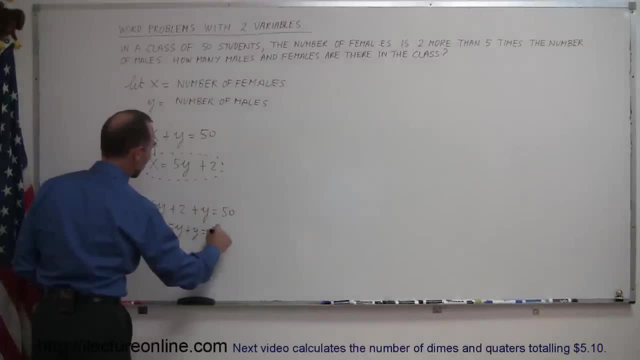 so 5Y plus Y is equal to 50.. 50 minus two. remember, when the two goes across the equal sign, the sign changes. Now we can combine like terms on both sides. So this is: 6Y is equal to 48, divide both sides by the coefficient in front of Y.